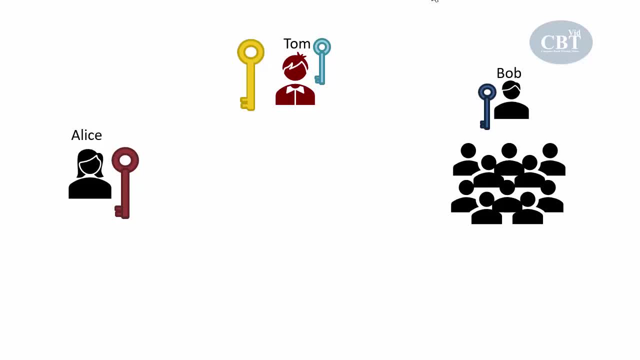 that that is Alice's public key. Now Alice wants to send a message to Bob. She encrypt that message using her own private key and then send that message to Bob. But then Tom plays man in the middle here and he stops the message. He decrypt the message using Alice's public key and then 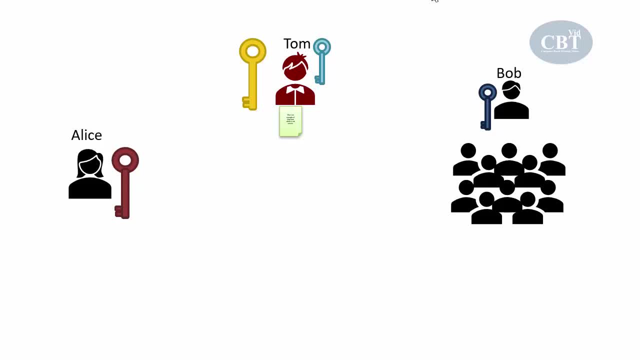 read the content of the message, changes that message to whatever he wants, and then he encrypts the message using his own private key. And then he decrypts the message using Alice's public key And then forward this message to Bob. Now Bob uses Tom's public key to decrypt the message. 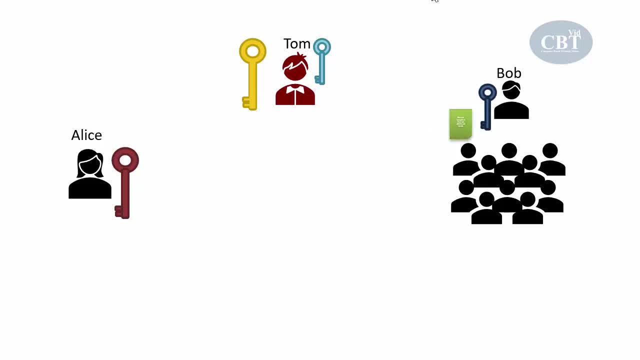 and see the content of the message, thinking that the message came from Alice. Now, this is a big issue. How do we address this problem? Well, digital certificate is actually an answer to this issue. Digital certificate is a technology used to decrypt messages, And it's used to decrypt messages. And it's used to decrypt messages. 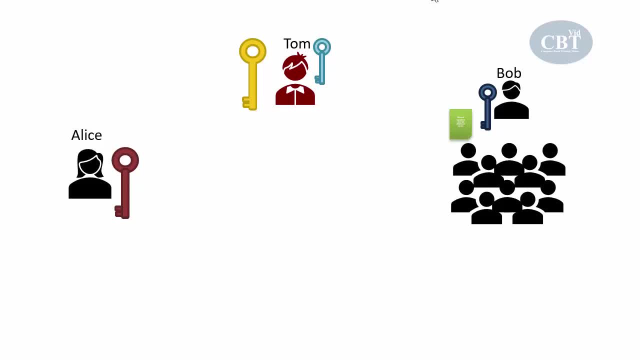 And the difference here is that digital certificate has laws. that says that you can tel l Alice's public key and send her a message to Bob, But in reality Bob doesn't do that, So this is not for our purpose If you use Alice's public key and you try to hide the message group. 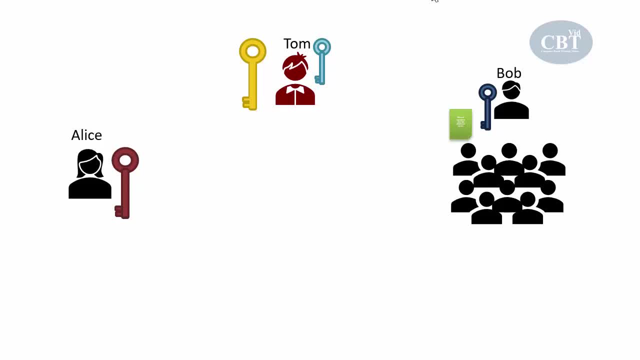 then you will respond. So you will be surrounded by the message group, but this notification sister, not the device for that. In reality, the message will be sent to Alice's public key. It's didnren now, But when you decrypt the message to these people using this digital certificate, at least an. 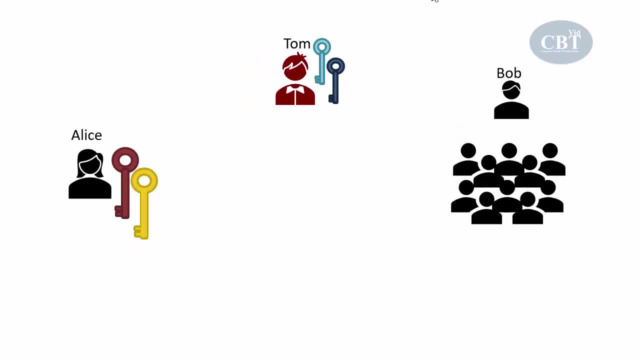 Xbox user will assume that you will send it to Bob Because you are using Alice's public key sign defunct, So you book by the browser, Crowdy out of them and release the message program So you use. Alice's concept is similar to the real-world identification cards that we have. Let's say, I want to withdraw. 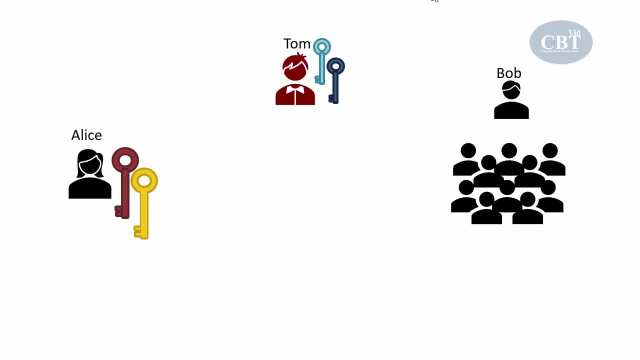 some money from my bank account. So I go to the bank and I tell the teller I want to withdraw some money. The teller asks me: please provide some identifications, because the teller doesn't know me and she wants to make sure that I am who I say I am, So that's why she needs. 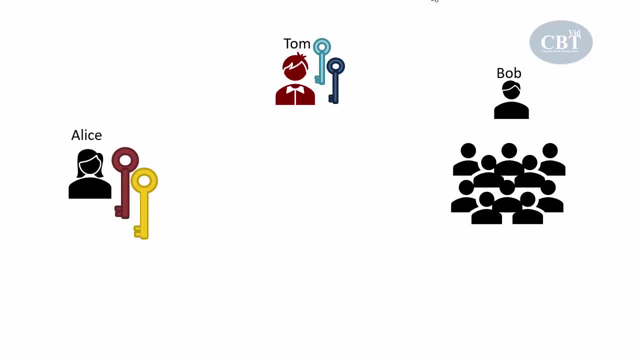 a piece of identification card. So I provide my driver's license and the bank teller accepts that driver's license as a proof of identity. Now here is a question: Why does she accept the driver's license as a proof of identity? Why doesn't she accept a piece of paper that? 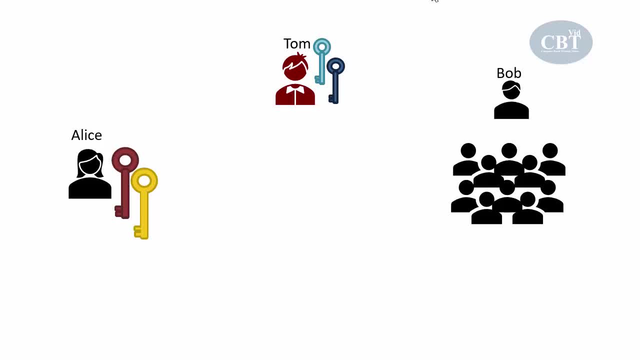 has my picture on it and right next to that I just write my name. Why doesn't she accept that? You all know the reason that she accepts that driver's license: It's because that driver's license is issued by a trusted party. It's a trusted government. 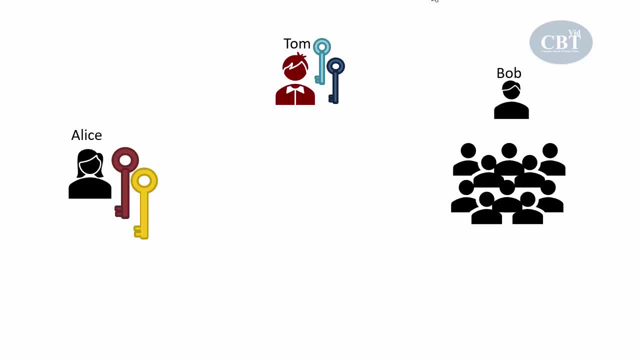 agency who issues that driver's license. That's why the bank, teller and anywhere else they accept driver's license as a proof of identity. Now, in the same way, digital certificate is issued by a trusted third-party agency, So that trusted third-party agency is called. 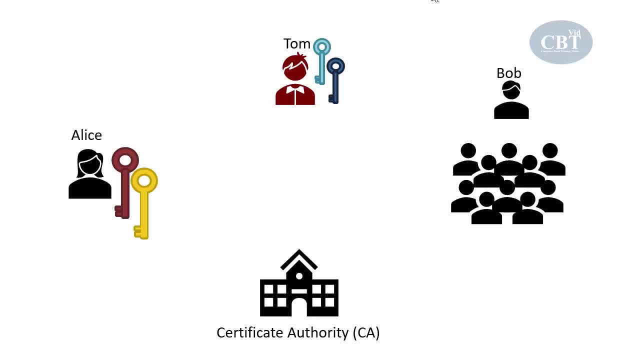 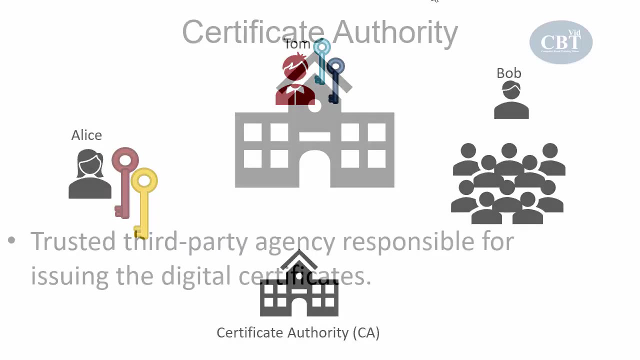 certificate authority. Here is a question. Here is how the whole concept works. When Alice wants to communicate with Bob, instead of sending her public key to Bob directly, she's going to send her digital certificate, which is issued by a trusted third-party. Now who is this certificate authority As? 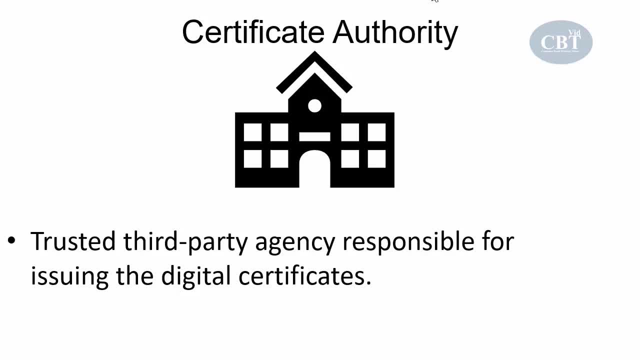 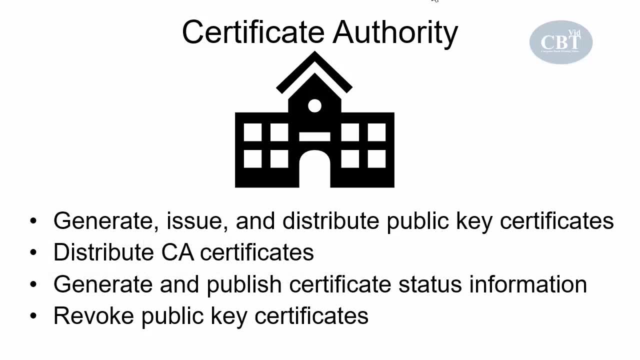 I mentioned, it's a trusted third-party agency that issues digital certificates. Now, in addition to issuing and distributing digital certificates, they also keep track of the status of the digital certificates, So you can refer to their website to find out if a certificate is valid or not. 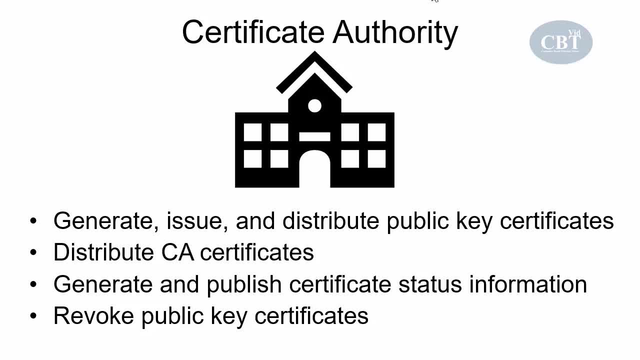 They also revoke public key certificates the same way that the Department of Motor Vehicle revokes a driver's license. So if you are doing a lot of driving faults, then your driver's license gets suspended or revoked. So that's basically the responsibilities of certificate. 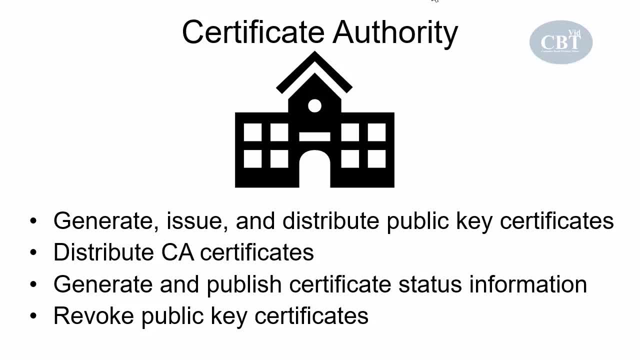 authority. Now, how do we get this digital certificate authority? Well, first of all, you need to get a certificate from a trusted third-party agency. You need to get a certificate from a trusted third-party agency. Let's say Alice wants to get a digital certificate. Let's: 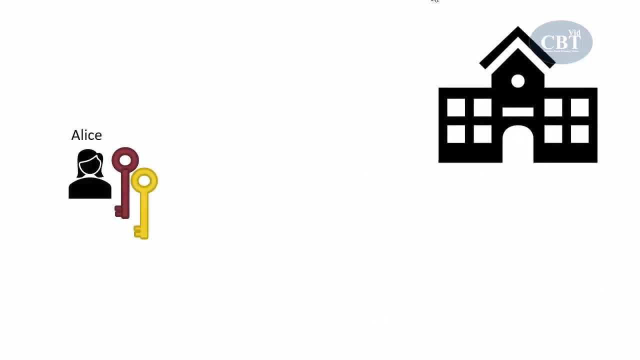 say, Alice wants to get a digital certificate. So what she does is she generates a certificate signing request. In that request she provides all the information that certificate authority needs. For example, she puts her website, her business name, the city, state, country. 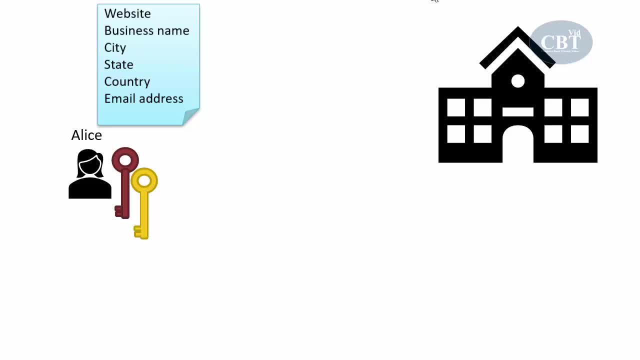 and email address in that request And she also provides some proof of identity like her passport or ID, And she also provides some proof of identity like her passport or any other identification card that certificate authority requires. She adds her public key to this request and then she forwards that to certificate authority. Then that certificate 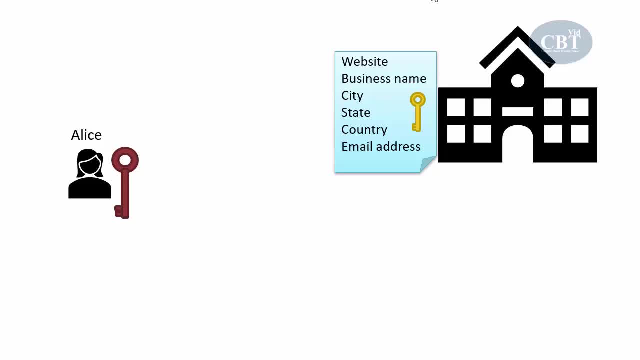 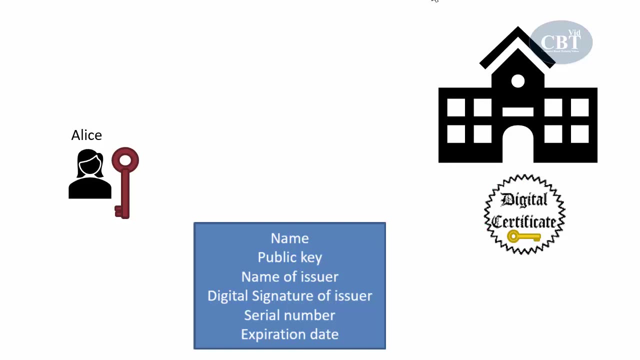 authority agency will verify all the information and the public key And, after all of that, they're going to generate her a digital certificate. Now in that digital certificate we have Alice's name, her public key and the name of the issuer, meaning the certificate authority agency who issues this digital certificate. 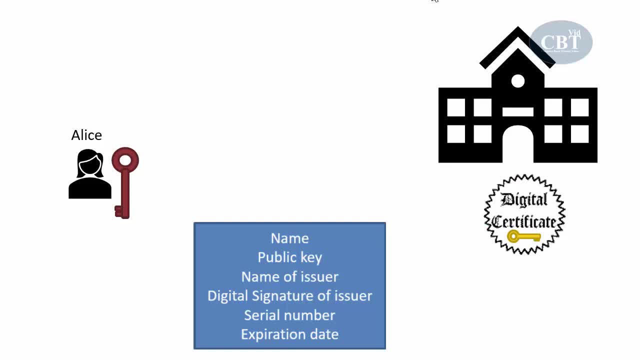 the digital signature of the issuer, the serial number and the expiration date of the digital certificate. All of these are inside that digital certificate. Now you may ask: why do we need to have the digital signature of the issuer? Well, I'll. 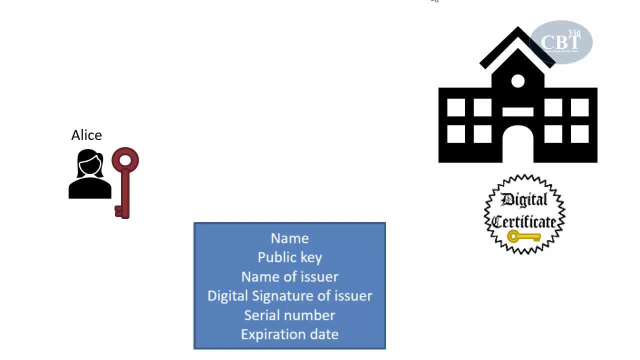 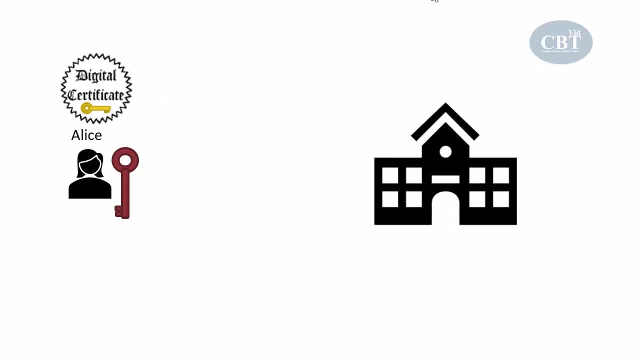 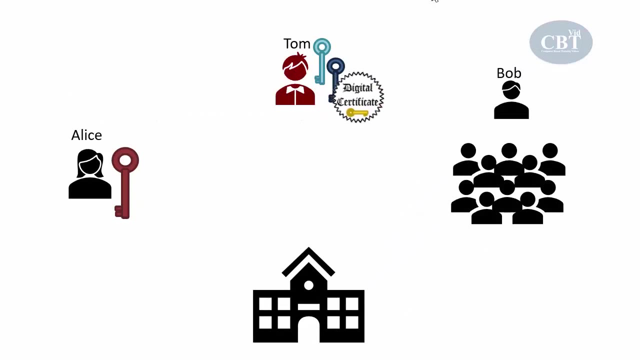 talk about that shortly. So now, once the certificate authority generates that digital signature, they forward it back to Alice. Now, from now on, when Alice wants to communicate with anybody, including Bob, instead of sending her public key to Bob, she sends her digital. 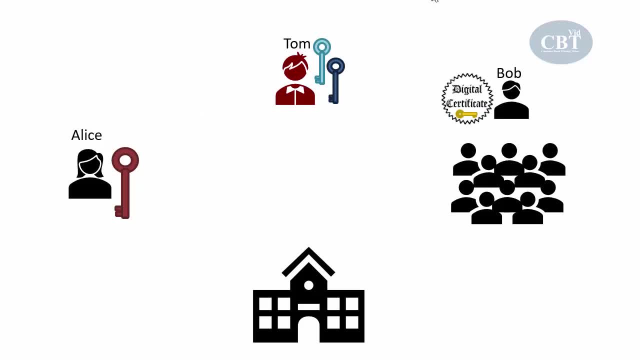 certificate. Now, when Bob wants to verify this digital certificate, he basically verifies that with that certificate authority agency And if the verification process goes well, then Bob knows that that public key is Alice's. The public key is actually Alice's public key and that certificate is actually Alice's. 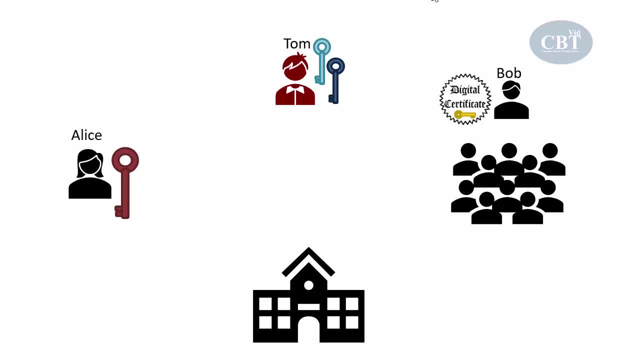 certificate. Now how does this process of verification happen? How does Bob verify that He's not going to send that to the agency for verification? What happens here is when certificate authority agency receives the certificate signing request from Alice, they're going to generate a hash of all the information there. 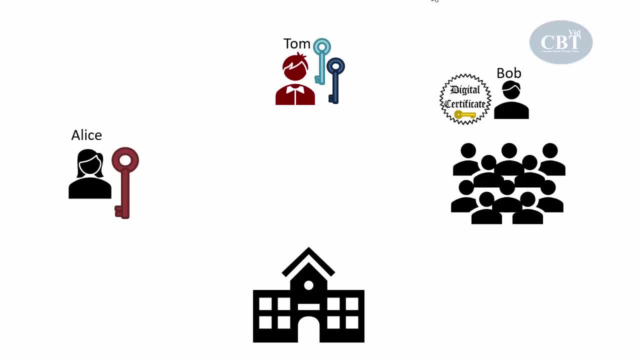 Using one of the hashing algorithm that we saw in previous video And then, once they have that hash, they're going to encrypt that hash using their private key. So now, when the hash is encrypted using the certificate authority agency's private key, only their public key can decrypt that. 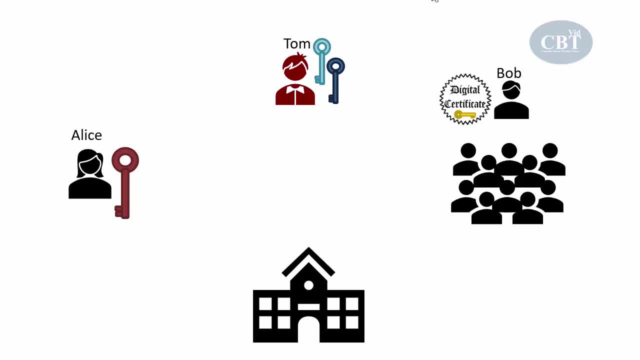 message. Now, when Bob receives this digital certificate, he's going to create a hash of all the information in there. Then he's going to go get the public key of Alice's private key. Now, when Bob gets this certificate, he's going to use the public key of Alice's certificate. 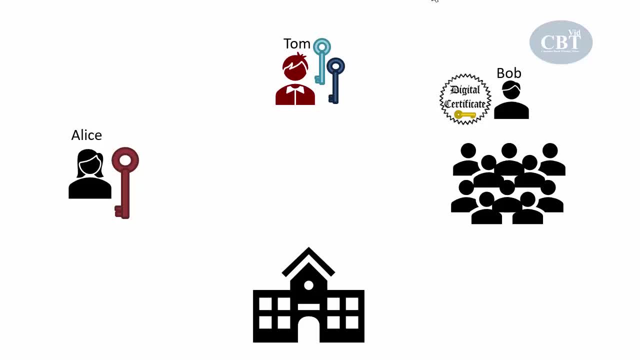 authority agency and use that public key to decrypt the hash that was encrypted in that certificate. If Bob can decrypt that hash, then he knows that that certificate was signed by the certificate authority agency that was mentioned in the digital certificate. Then he's going to compare this hash with the hash that he created earlier. If these 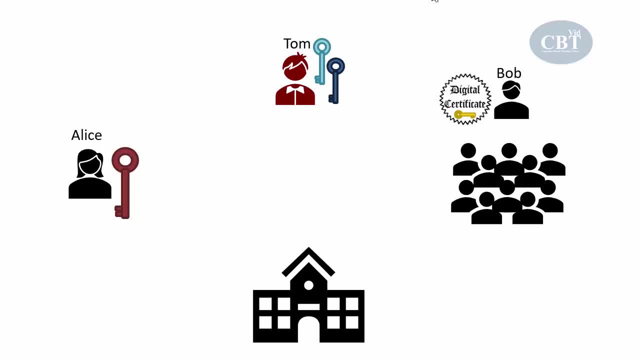 two hashes are the same, he knows that he has to decrypt the hash that he created earlier. same then. bob knows that this digital certificate is a valid certificate and it was actually signed by the certificate authority that was mentioned on the digital certificate. now, even if tom in 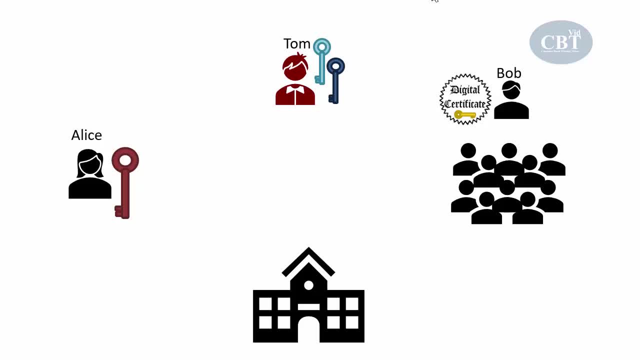 between tries to steal that digital certificate and change the content of the digital certificate and send his own public key with a fake certificate to bob, then when bob tries to verify that digital certificate, the whole verification process is going to fail because bob is going to use the certificate authority's public key to decrypt the whole message and then 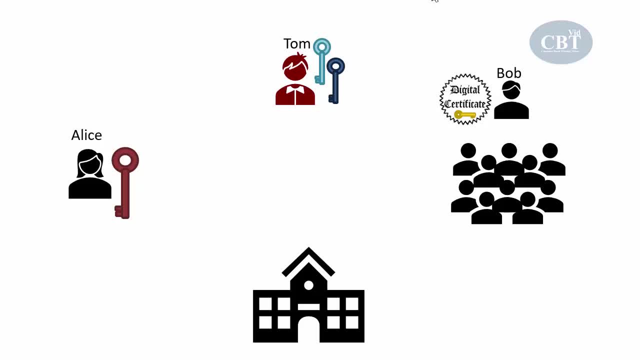 when he uses that certificate authority's public key. the decryption process is going to fail and bob knows that this digital certificate that he's received is not actually alice's digital certificate. all right, now that we know the concept, let's go and take a look at an application. 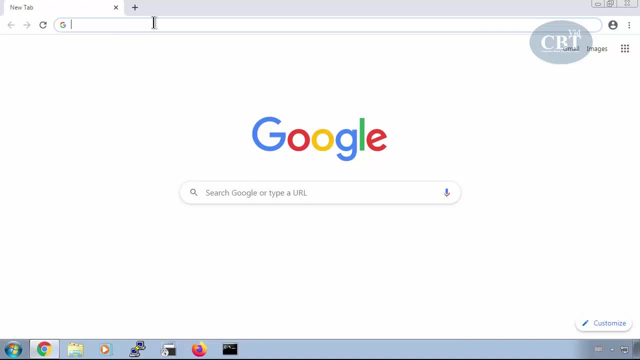 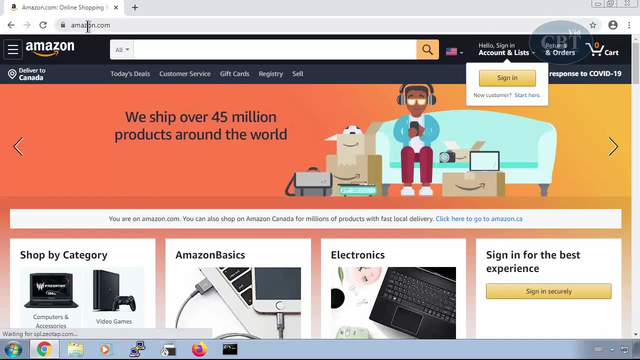 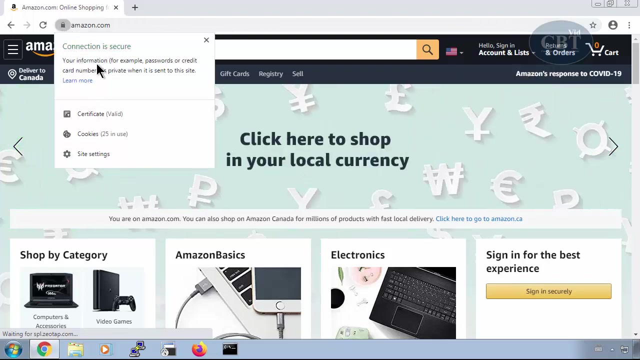 of this digital certificate. let's say you want to do some shopping and you go to amazoncom. so when you're on the website, right here next to the url that you see- amazoncom- we have a lock. if you click on that lock you can see here it says the connection is secure, and down here it. 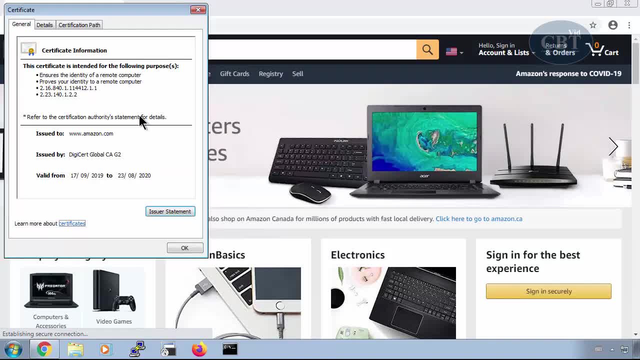 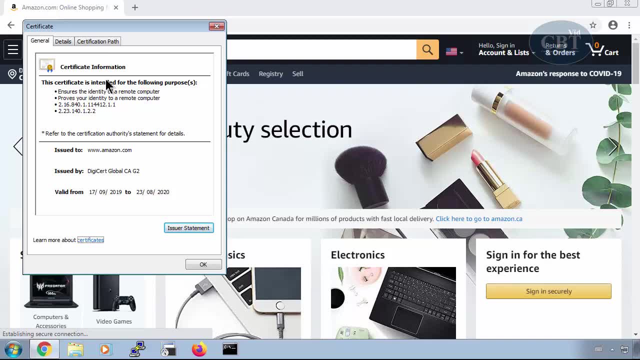 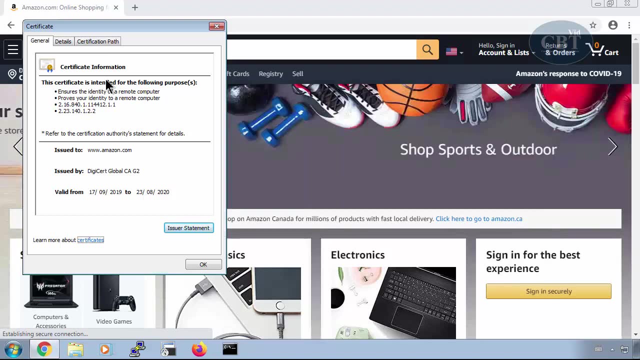 says certificate is valid. so let's click on that and here we have some information about the certificate that we have received. so the whole certificate exchange that we saw between alice and bob here it happened between my web browser and amazon's web server, so these two were actually doing all those certificate. 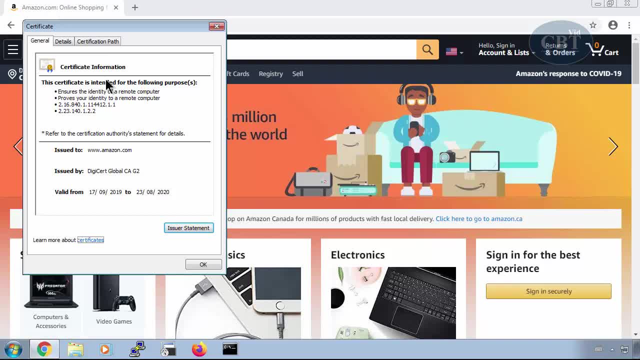 exchange and certificate verifications. so in this concept, amazon's web server is alice and my web browser is bob, so bob, who happened to be my web browser, received this certificate. now here are some information about this certificate. you can see it says the certificate has been issued to. 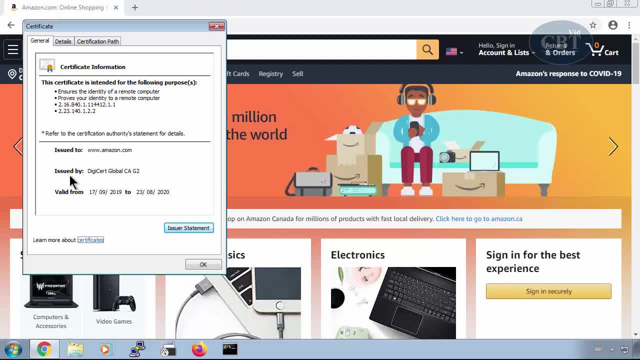 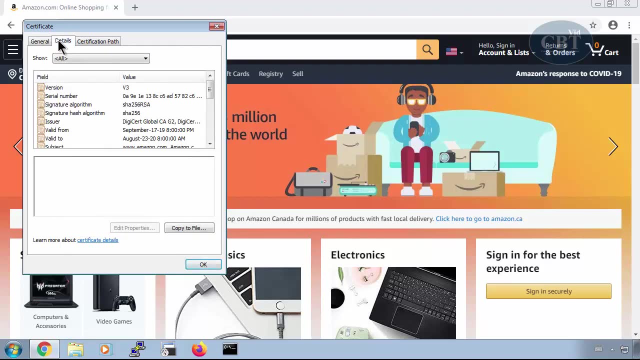 amazoncom and the certificate. the issuer of the certificate or the certificate authority organization is digi cert global cag2. the certificate is valid from this state to this date and if i click here i have some detail on that certificate. you can see the version of the certificate, the serial number of the certificate. 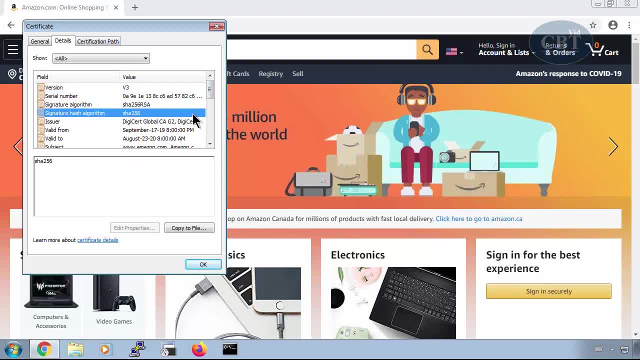 here is the signature hash algorithm that was used, that's sha256. the issuer: the valid from and valid to. and here is subject: information and down here you can see it says: this is a website, the organization is amazoncom incorporation. the location, the city is seattle. the state is 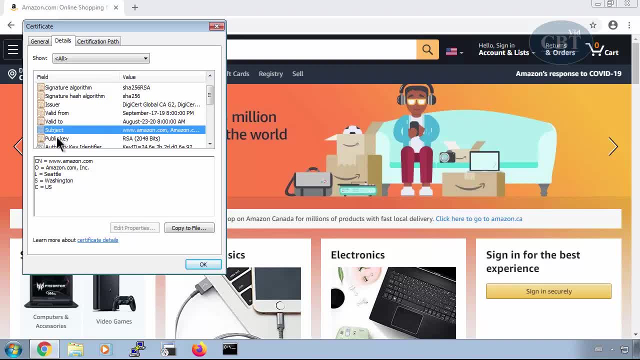 washington and the country is the united states, and here is the public key. so you can see a public key was included in the digital certificate, so my browser receives this information and then it verifies that with the certificate authority and that's one application of digital certificate on internet.